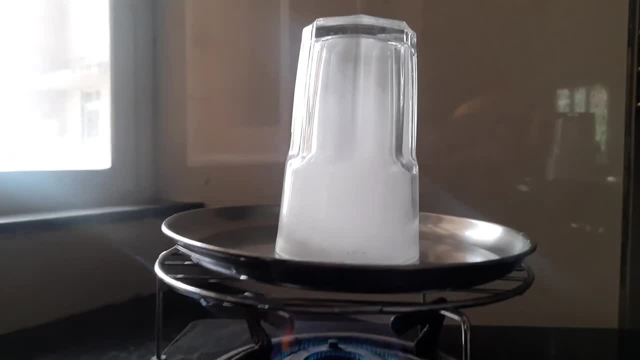 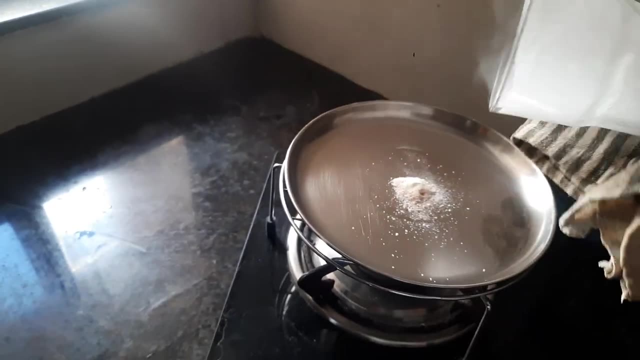 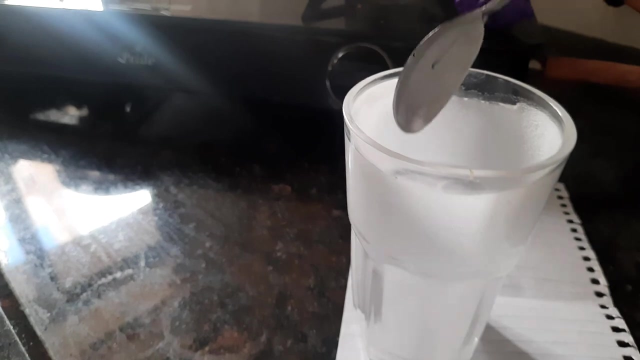 state. We have camphor, some of the camphor- in its vapor state, and salt is still solid. So now if we take away the glass, we will have to be very careful here. We can let the glass cool for some time, And when we do that, notice what happens. We see this white substance being deposited on the 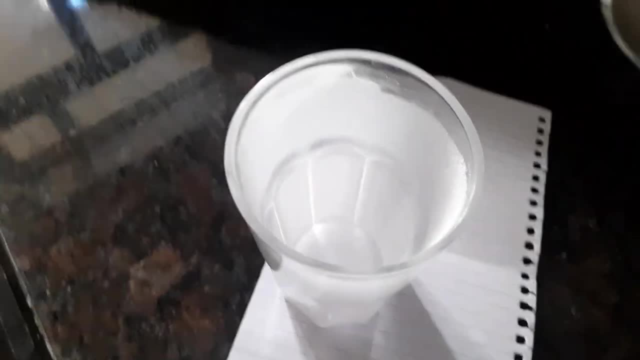 walls of the glass, right? What is that? Well, that's camphor. Camphor vaporized, And once the glass was allowed to cool, it was able to cool down. So now we have camphor, And when we do that. 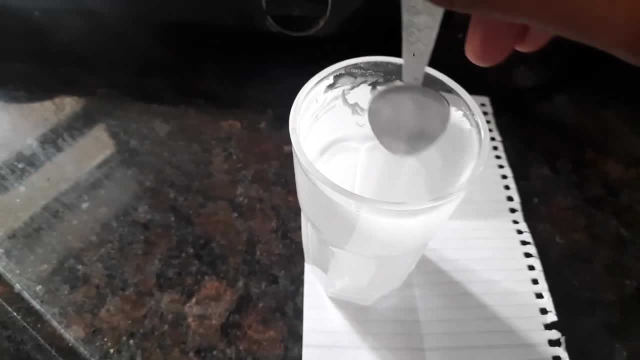 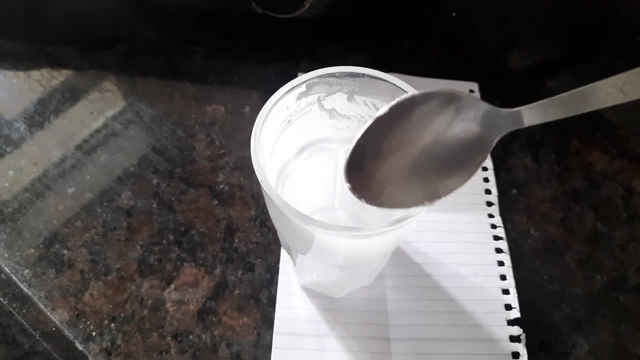 we see this white substance being deposited on the walls of the glass, right? What is that? Well, that's camphor. And once the glass was allowed to cool, the camphor turned back into solid state And we can see camphor being deposited on the walls. Just have a look at this. This is camphor. 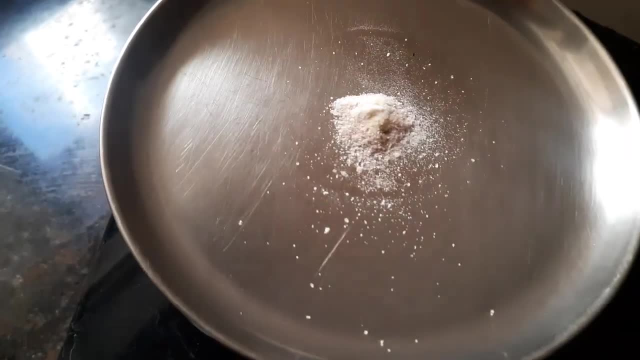 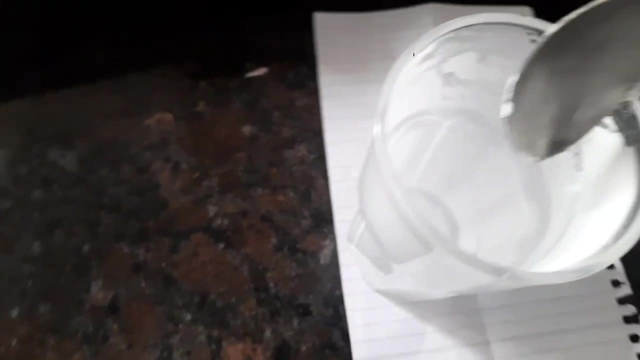 If we look at the plate again, we will see the salt present And there will be some camphor as well, because we did not let all the camphor change to vapor. So from the process of sublimation we were able to separate camphor from salt, a mixture of camphor and salt. Camphor turned. 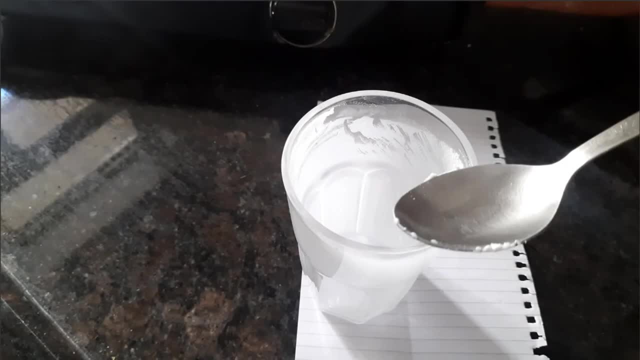 directly from solid to vapor. That's called sublimation. And once the glass was allowed to cool, once it came into contact with the walls of the glass and the walls of the glass were given some time to cool, camphor changed back to solid form, And that is what we see on the walls of the 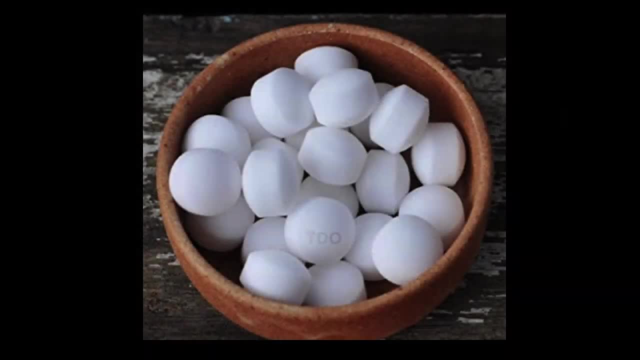 glass. This is quite cool. Now you must have used naphthalene balls right. Naphthalene balls are used between clothes to repel moths and other insects that can damage fabrics, And naphthalene balls they directly turn to gas, just like camphor. And when they do change, 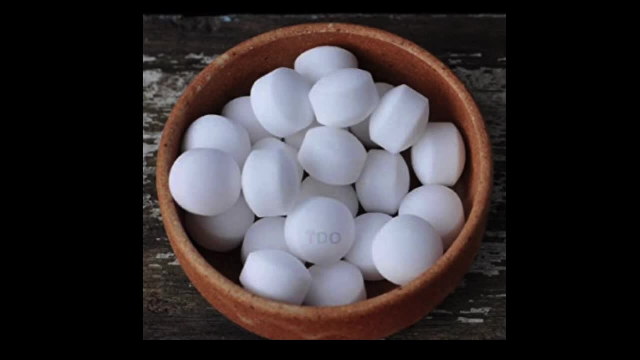 to gas. that gaseous form of naphthalene is toxic to insects, And this gas spreads throughout the surrounding area, creating like a protective barrier around the clothes. So this shows that science is really all around us, even in the simple things we use every day, like naphthalene. 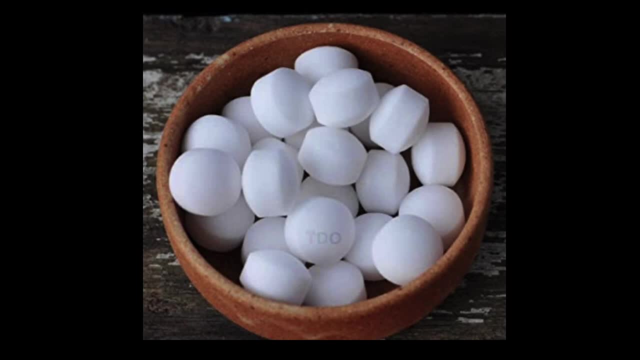 balls. It's amazing how the process of sublimation can be can be used to protect our clothes from insects. Science truly is awesome and can help us solve everyday problems in innovative ways.